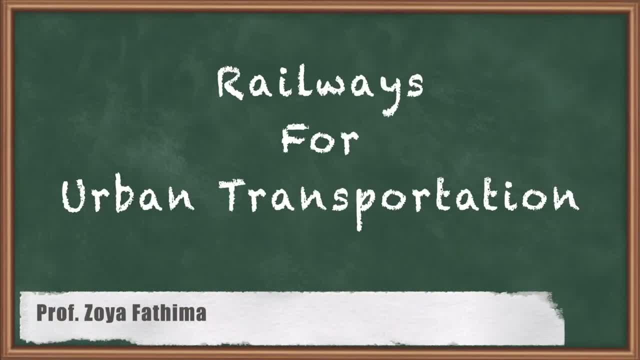 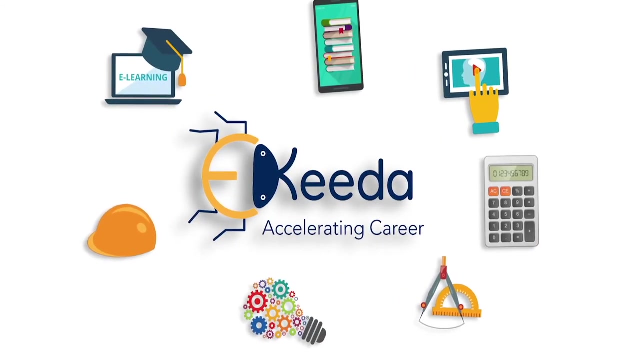 In this lesson let us study about railways for urban transportation. So firstly, we'll see what is urban transportation, how railways are interrelated to urban transportation and what are the different types of urban transportation in terms of railways. All these things we'll be studying in this particular lesson. So to get started with transportation management is a 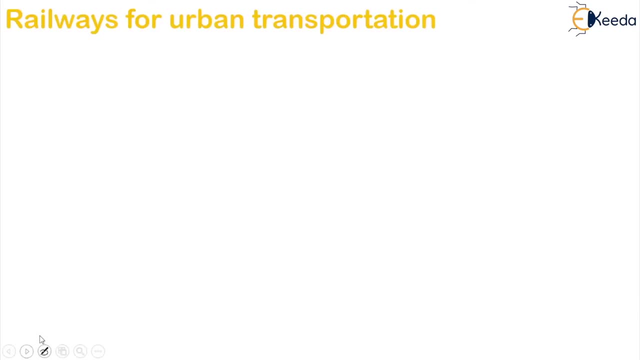 major part of urban planning and development. So urban areas worldwide are rapidly expanding and also the urban population is also expanding. Urban is nothing but big cities or metropolitan cities. So urban planning majorly impact how much city supports your business growth, or of which transportation management has a key role to play. So city transportation influences. 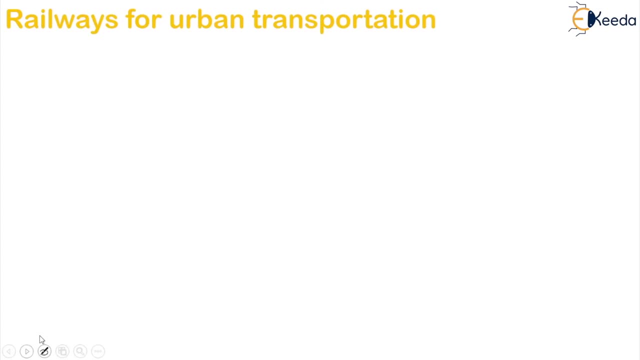 what per capita expenditure is. So urban planning is a major part of urban planning and development, So to a large extent that the country's GDP Normally due to sudden increase in the urban population, typical man hours spent on the traffic in a day or traffic hazards and the population. 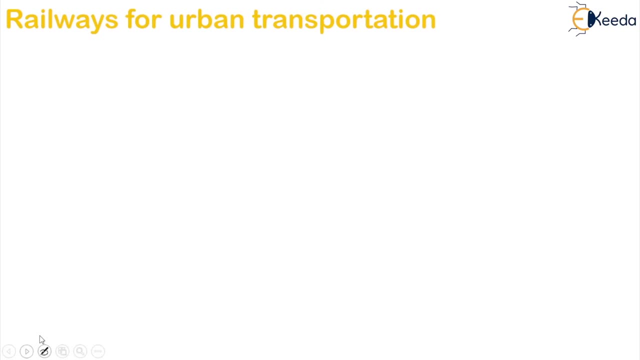 level. all these things are dependent upon the traffic mode and the sizes in the city. What is the size of the traffic and what is the mode of the traffic? on all these things it will depend. So, additionally, the pride value of urban transportation is a major part of urban. 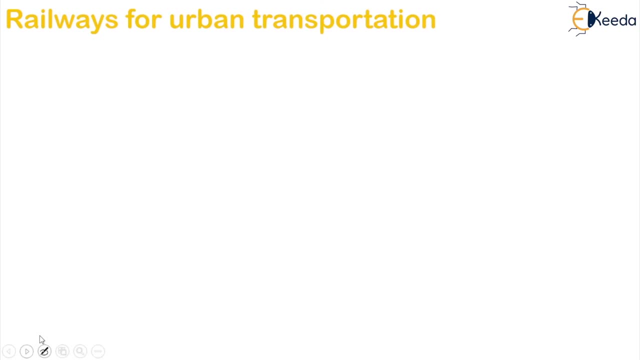 planning and development. So urban planning is a major part of urban planning and development. So additionally, the pride value of urban planning and development, So the pride value of the city and the country, lies with the traffic behavior along with all other factors. Now in many urban 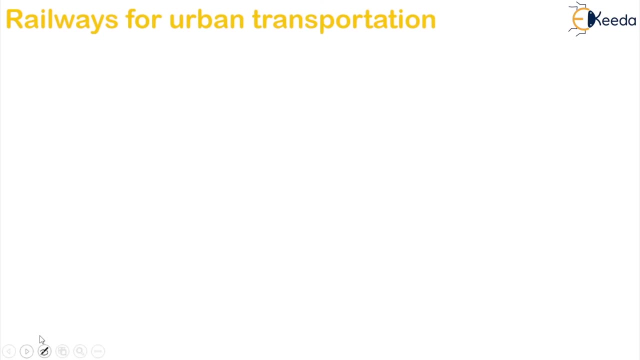 countries, railways are used as the means of transportation to move within the city, So there is a lot of urbanization when it comes to railways, especially when the movement is within the city. So the advantages of using railways is: railways are your mass transit system. So why are we? 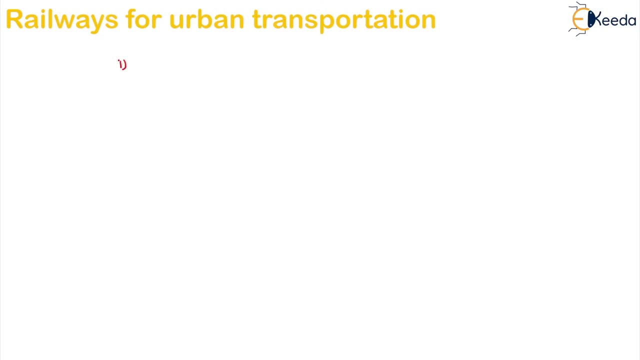 using railways for urban transportation, one reason being what it is: a mass transit system. A lot of people can travel in one train, right? So if you see the example of Mumbai, Delhi and all urban countries, railways will help for mass transit system. Hence what will happen? it will be more efficient. 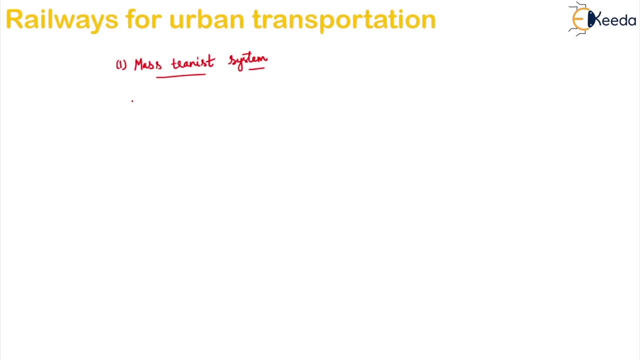 than your roadways and it has higher land based traffic capacity demand Right. Also, railways has high capital intense use when you compare to other modes of transportation. so highly, highly capital incentives and railway transportation requires a very long time for your planning and take it. 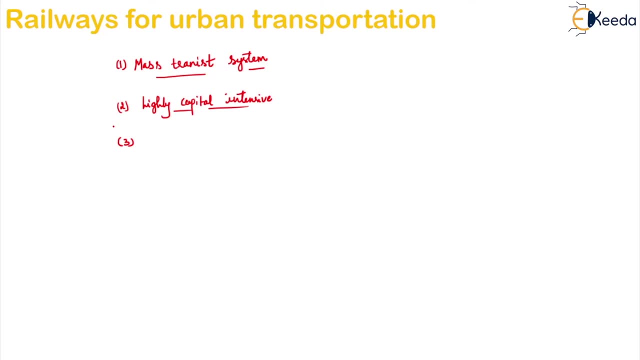 will take years to design, develop and build the infrastructure of all the things, but it will cause minimum impact for the existing structure when it is properly designed. so long time for planning. so all these are the major concerns of your railways for using it for transportation. right now, there are different types of railways which we see in the urban transportation. so, in order 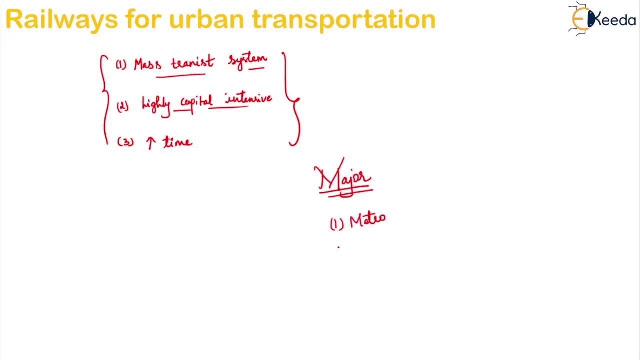 to list out few. the major ones are metro rails, light rail transit, lrt, also called as what light rail transit right, and the third one is the mono rail. so these are some of the major or important ones. if you want to the list of all the types, here they are: the tram, light rail, rapid transit, monorail, metro. 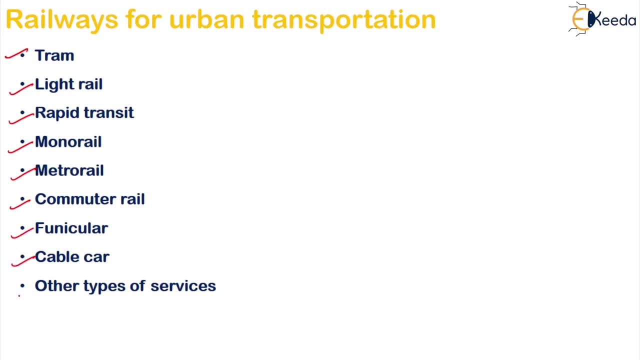 rail, commuter rail, funicular, cable cars and some other types of services also. so these all will come under the urban transportation category, specially in your railways. so let us see one by one, on what are these see? basically the thing is, the urban rail transit is an all comprising terms of various types of local rail systems providing passenger service. 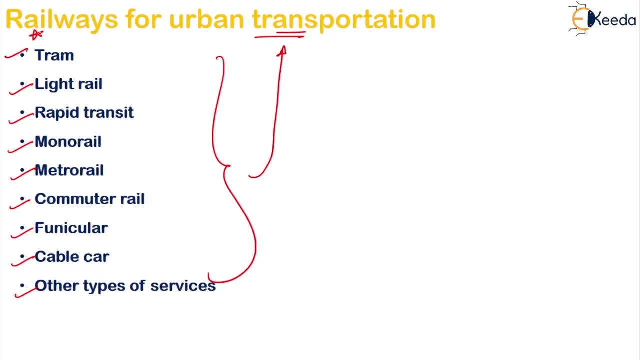 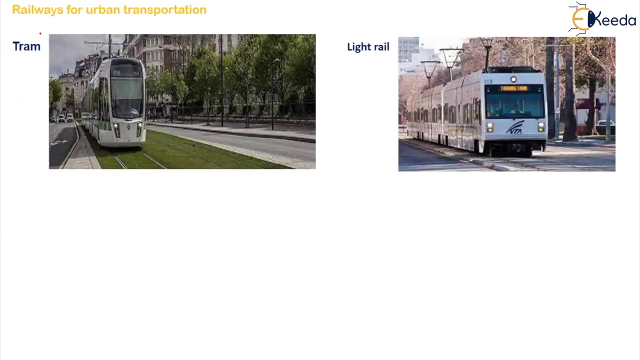 within and around the urban and suburban area. so the set of urban rail systems can be roughly divided into these all categories. in some places there may be overlapping of categories also, right. so let us see one by one, what are these types? so the first one is your tram. 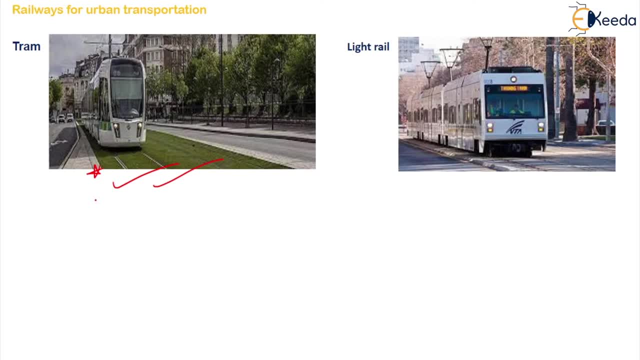 you can observe here, this is your tram. so these trams are also in few countries. you can see, the trams are also in few countries called as street cars or trolley systems, and these are rail based systems that run mainly or completely along the street. so, if you can, 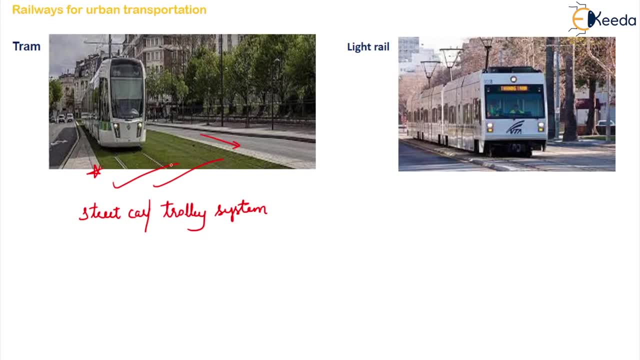 observe there is a street here and along the street these will run, so these have very low capacity and very frequent stops. normally what will happen is the passengers can board into this on the street or the crub level itself or on the low floor level itself. so 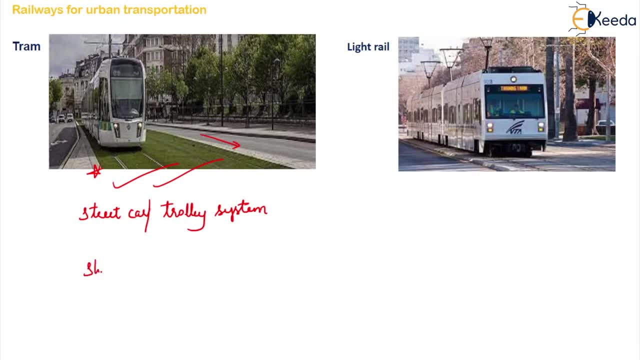 I do see that, see how people ride them, how these trams operate. I show, for instance, in a long distance line right, these might be of short distance also and these might be of long distance also. certain long disc trams are called as introubance or a radial rails. 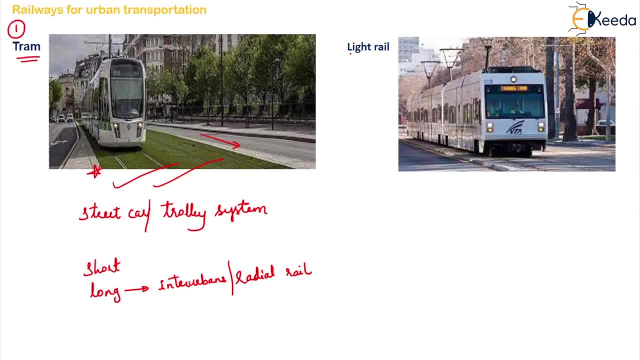 are called radial rails in India. you can see this in Kolkatta, right. so these are your trams. second one is your. so a right rail is a rail based transit, same like your tram, but these have a higher capacity. you, we didn't note it, so here, if you want to note, it has low capacity and frequent stops, right. 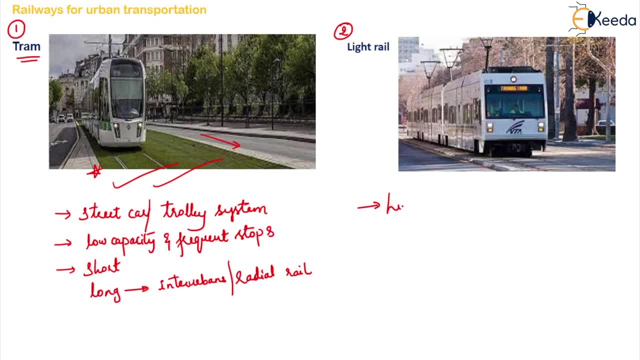 whereas in case of light rail it has higher capacity and also they run in a speedy manner. so these are of low speed. trams are of low speed, whereas light rails are of a higher speed, usually by operation in an exclusive right of way, separated from the automobiling traffic, but which is not. 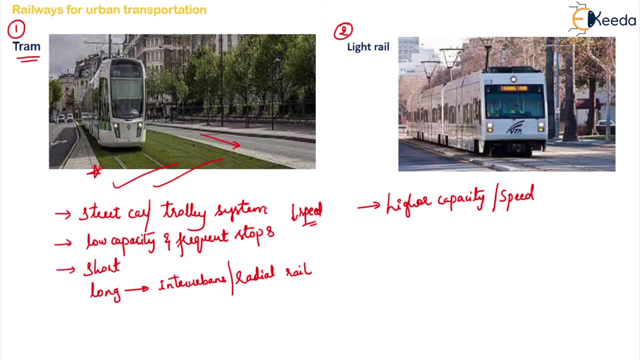 fully grade, separated from the traffic right. so in between your traffic it will try to move. so light rails are also generally operated with multiple unit trains. rather than your single tram car, in tram car there will be only one unit, whereas light rail will have many units right it. 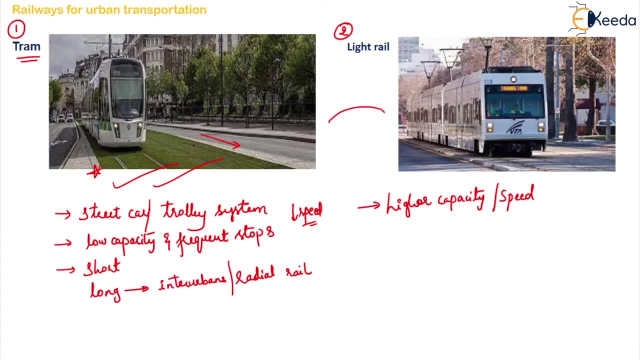 is one of the emergent or a better way, better version of your trams. okay, so for speed and capacity it is normally called right rail system. understood, there might be some crossings, level crossings also in this particular type of rails. so in india your chennai metro can come under your light rail. 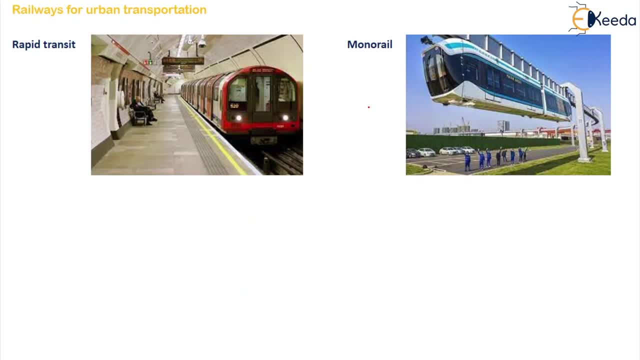 system. okay then, moving to the next one is your rapid transit. third one is your rapid transit. so this is a railway which is usually seen in your urban area, with high passenger capacity and frequency of service. so where will you normally see this? high passenger capacities and frequency of service, and usually 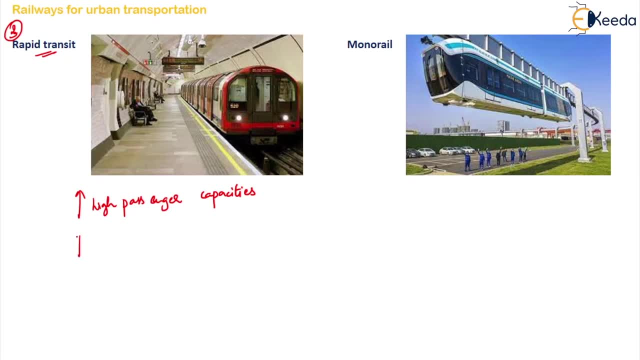 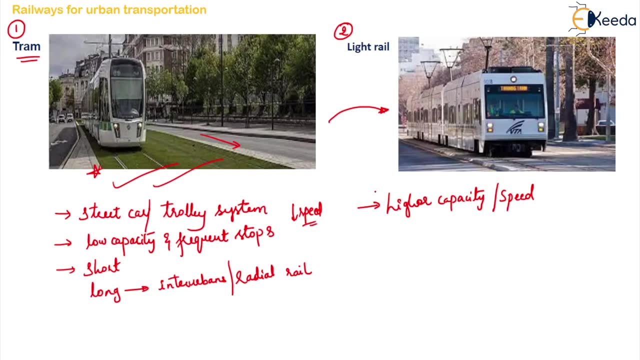 full grade separation from other traffic. here there will be full grade separation. full grade separation normally what will happen in the previous two? there is no full grade separation, there is a partial grade separation. means what there might be traffic, road traffic which is beside these, only your road traffic will be run by the traffic which is the traffic, which is the traffic which is the 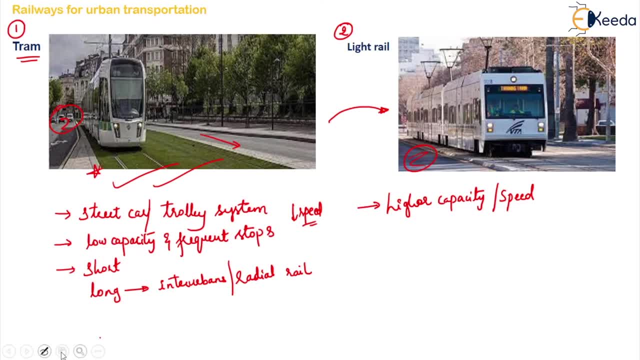 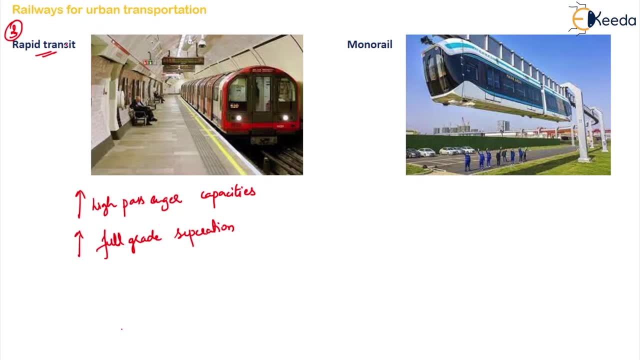 running, so there is no separation between a rail traffic and a road traffic, whereas when you come to your rapid transit here, it will be fully separated from your road traffic. okay, it's also called as heavy rail- heavy rail, so exactly opposite to your light rail. okay, in most of the countries this is 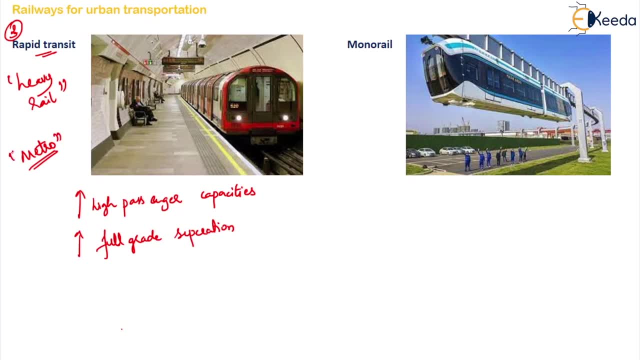 called as metro. the name for your rapid transit or heavy rail is your metro, because it comes in metropolitan cities, or they sometimes call it as metro. so this is called as metro. so this is called as your subway. also, in few countries it is called like this. some might be underground, they name them. 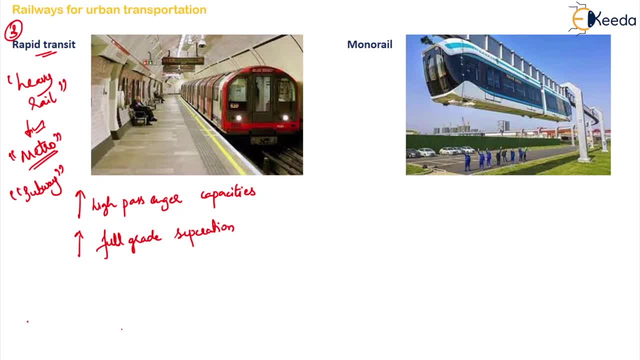 as tube right in chennai and singapore they are called as mrt mass rapid transit. so many countries have different names, their own names, for your rapid transit, but these are generally what for high passenger capacity and they're fully separated. now next one. the fourth one is the mono rail mono. 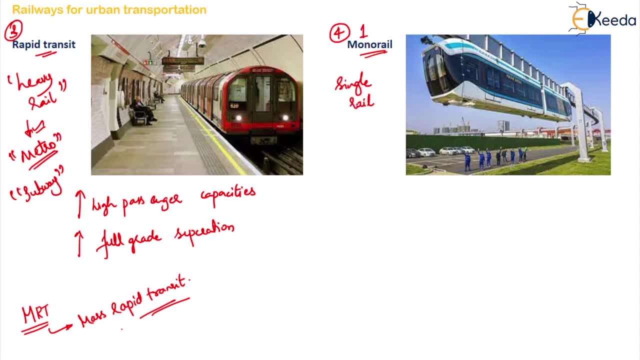 is what single mono is not a single rail. it is a single rail. it is a single rail. it is a single rail but a single rail, normally in a traditional railways. if you observe, in traditional railways you will have many rails right, many rails like this or many tracks like this right in mono rail. 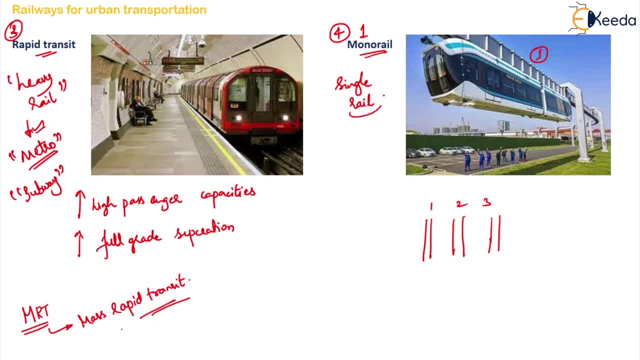 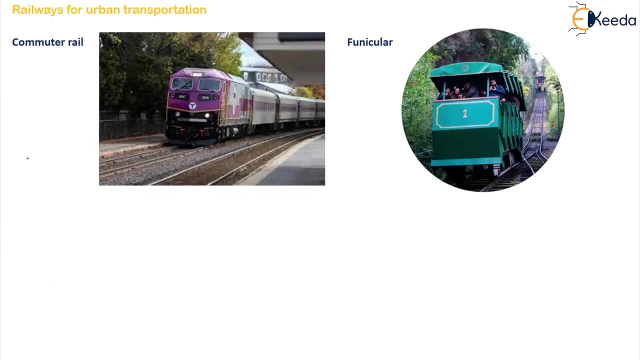 you will have only a single rail, and here modernization has occurred, so this type are called as mono rail. next is your commuter rail- see the other names for commuter rail. is your regional rail or your suburban rail, so these are the other names for your commuter rail. so these system operates on a main line trackage, which may be: 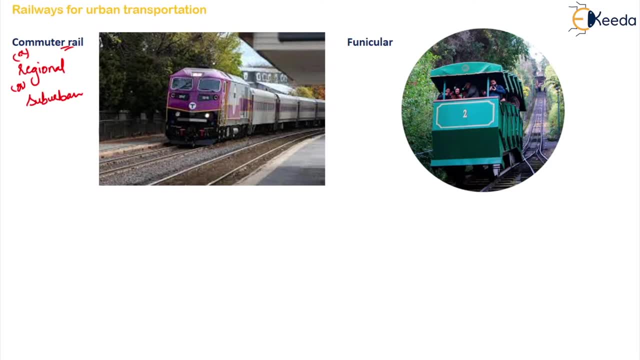 shared with intercity rail and freight trains, so these are between two cities. these are normal types of rails but between two cities, so system tends to operate on a low frequency than your rapid rail transit or your light rail system. but these will travel with high speed and has 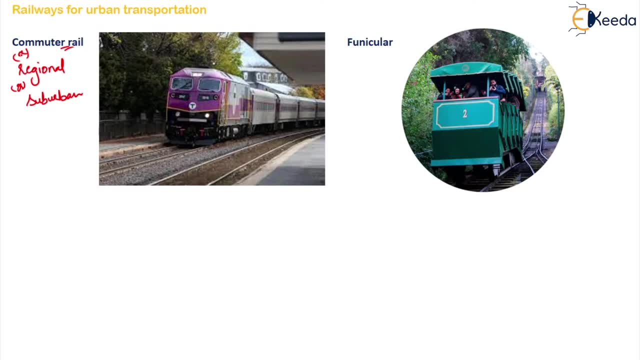 more widely spaced stations and will travel with high speed. and will travel with high speed, cover long distances. so these are lower in frequency but high speed, more space stations right, cover long distances. so this is all about your commuter rail. so this was the fifth one. next, the sixth one is your funicle rail. so it is this type of rails: are cable driven. cable driven- these. 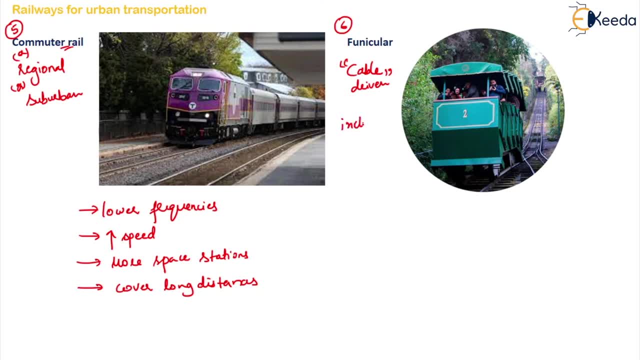 are normally inclined railways right. only in inclined the regions you can see this type of funicles. these type of rails will use the weight of descending car to help pull the ascending car right. the weight of one car will be used for pulling the other car is nothing but this. 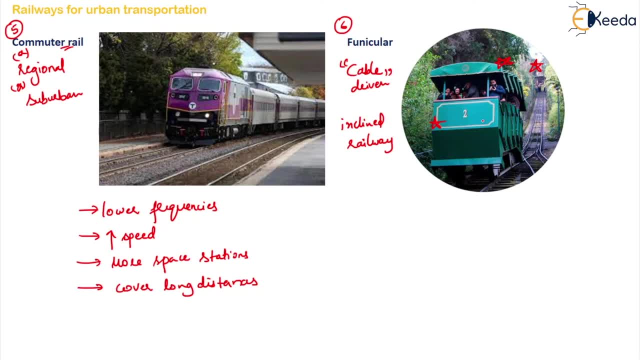 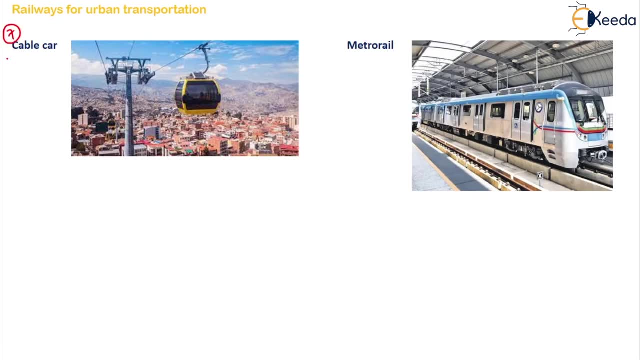 train bogey, or the portion of the train which has to be pulled, understood. so this is nothing but your funicle. next, moving on to the cable cars: so similar type of funicle is nothing but the cable car, but again, this is under your mass transit and uses the rail cars. so these type of cars are called what rail cars these can. 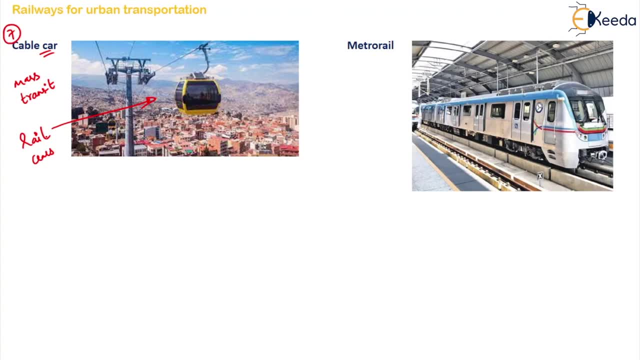 continuously move with a constant speed. they can move and individual cars can start and stop by releasing and gripping the cable as required. okay, so cable cars are distinct from funicles. distinct means separated in a way that in this cable cars the cars are permanently attached to your cable, but in funicle we can remove them, the vehicles can be attached and 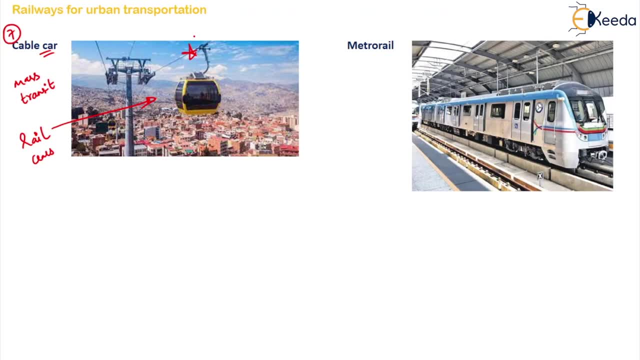 detached manually. so that is the major difference between your funicle and the cable cars, the last one being the metro rail. now, this is the major ones which you can see in India. right? so these are replacement of your what regular rails? they run on electricity, right? so in most of the cities,